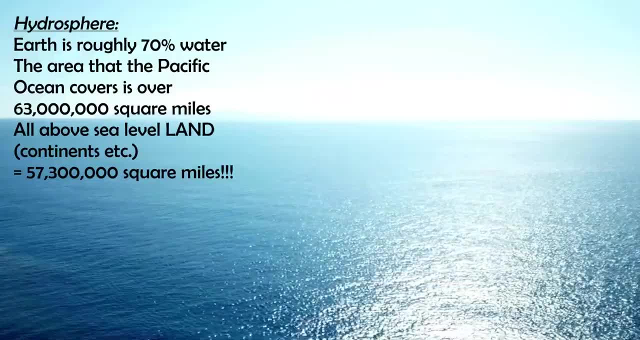 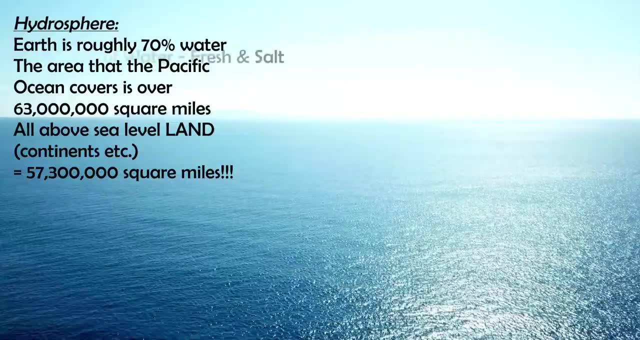 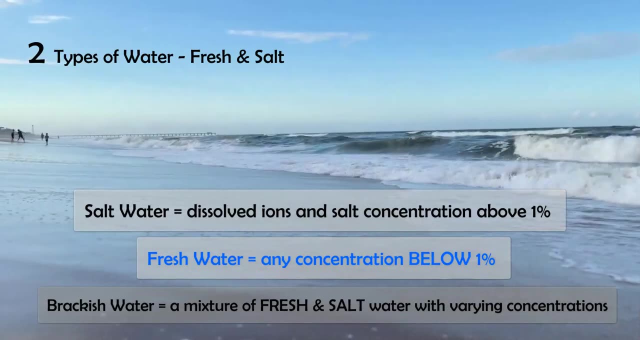 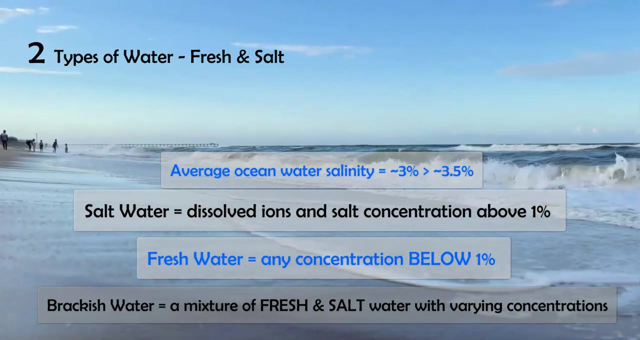 The planet is 70% water, 30% land and that also includes some of the cryosphere and frozen water. So it's a huge expanse, massive subject. let's delve into it Now. there are two types of water on this planet. There is the freshwater, which is rivers and streams and on the land, and you also have saltwater, which is around 1% average salt concentration and ions in the water that makes it salty. 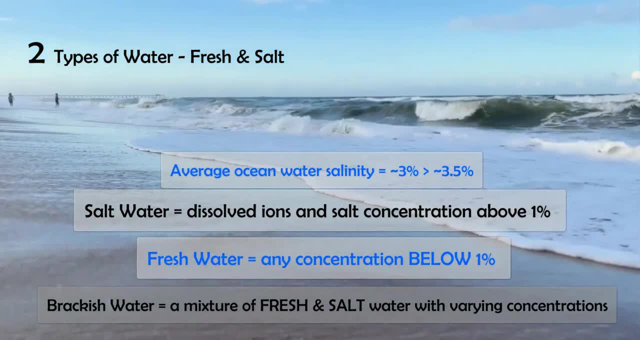 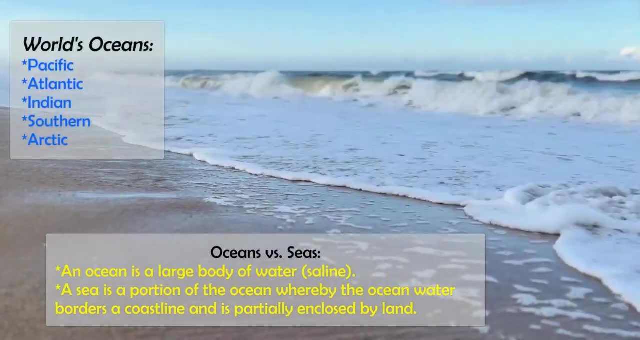 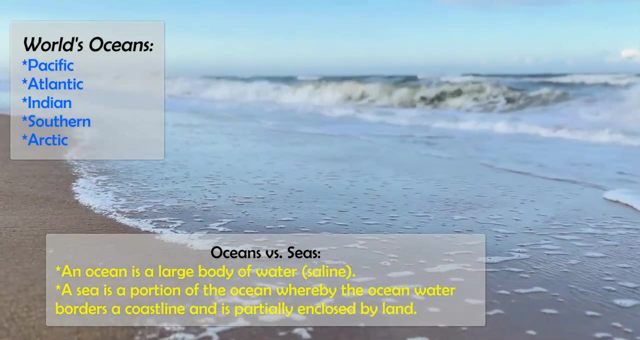 Now it can go as high as 3.5%, but the average is around 1.5% to 2.5%. so anything above 1% is classified as salty. So the oceans, the seas and this large expanse of water is the saltwater and we have certain characteristics compared to the freshwater. 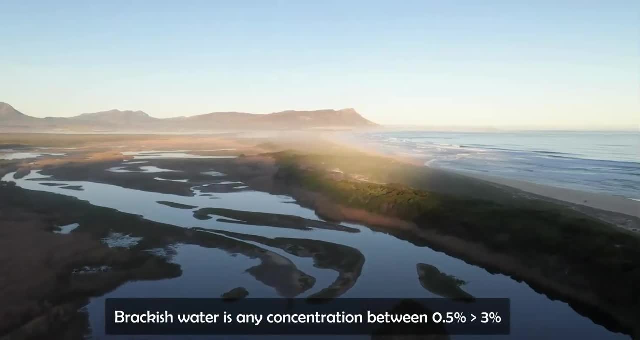 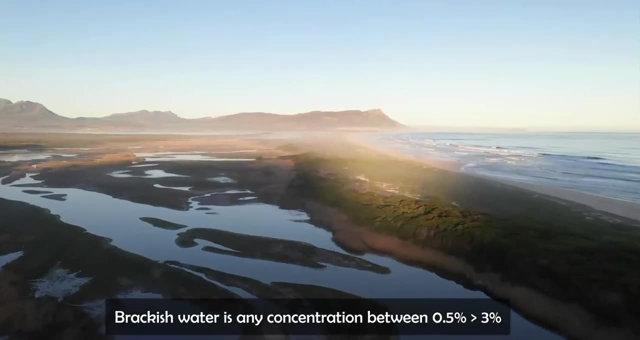 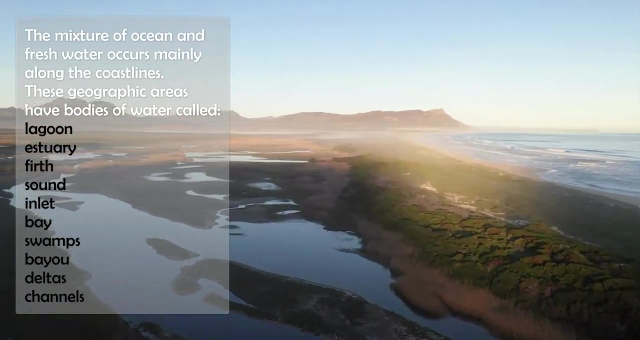 So from the oceans and seas, which are very large boils of water sitting on top of a solid ocean or sea crust or floor, you have the water that's on the land, on the continent, on the land masses, Anything above sea level. 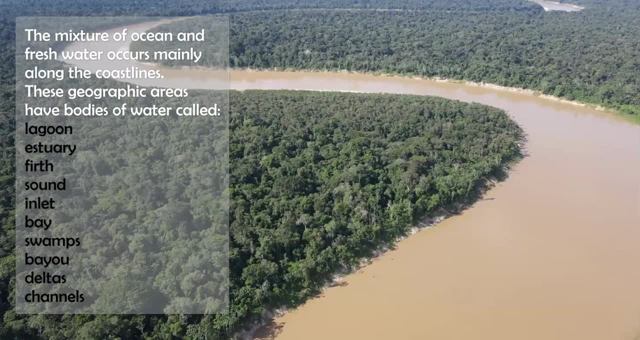 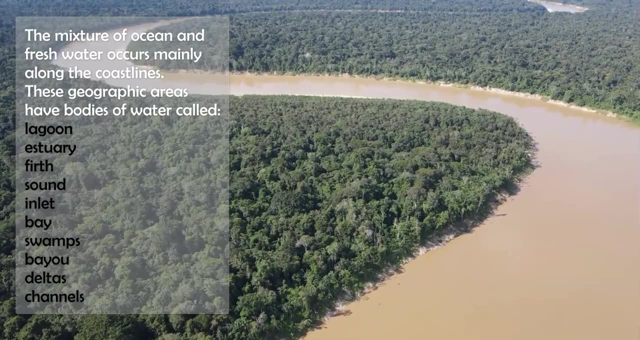 So you start with the coastal areas of estuaries, lagoons, wetlands, marshes, swamps, bayous, sounds, inlets, any kind of combination where the ocean is going to meet the fresh water coming off the land, and that's also called brackish water, which is a change of salt concentration. 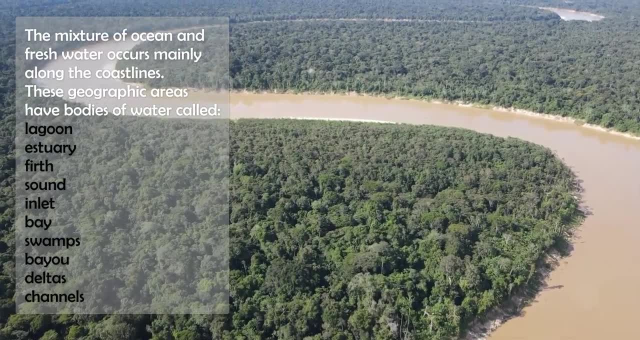 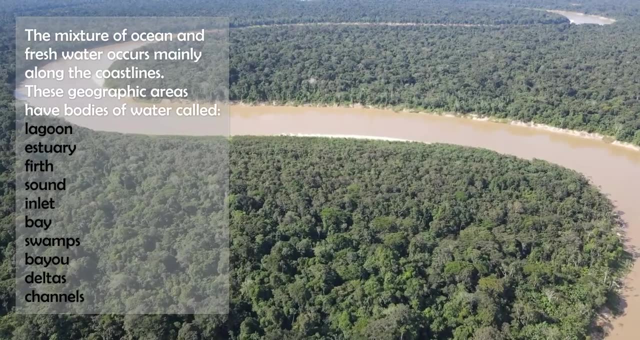 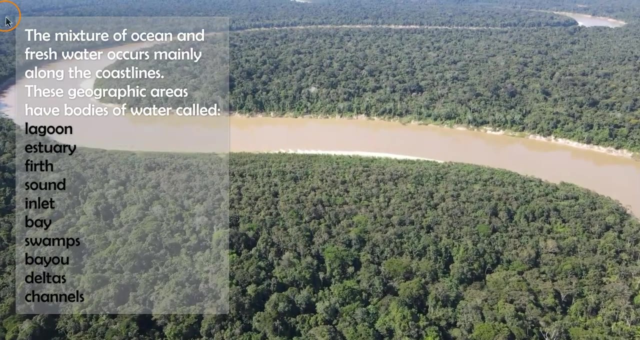 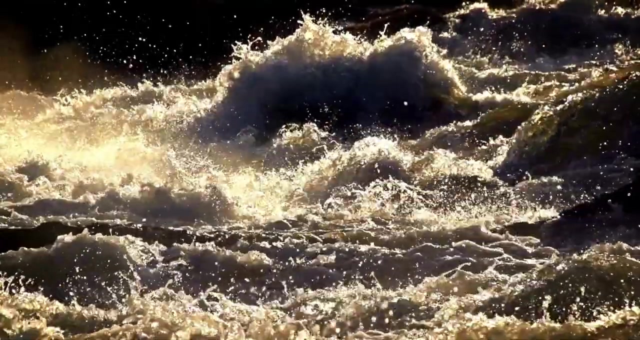 Then you get the beautiful rivers, the systems and watersheds and drainage basins of rivers flowing through the landscapes, over the landscapes, changing the landscapes and caused by the force of gravity forcing the water downwards towards the ocean. So, based on the amount of water flowing down with gravity over the Earth's surface or even through the Earth's surface, like infiltrating through soil and rock layers and different levels of porosity. 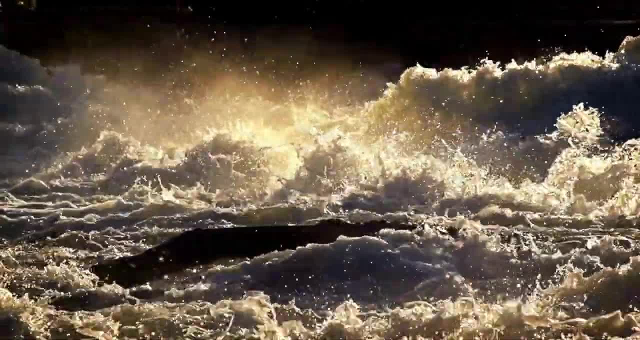 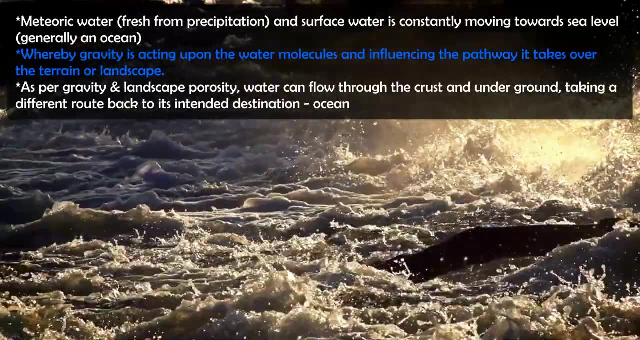 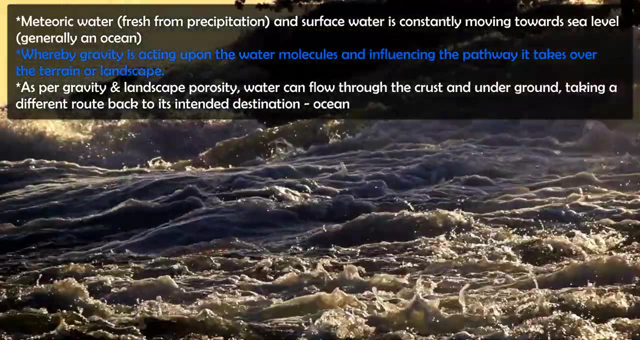 and permeability down to groundwater and flowing down through the ground back to the ocean, back to sea level. you have these different variations of rivers. you get from tributaries to brooks, to streams, to these large roaring rivers like the Amazon, the Ganges, the Mississippi, the Danube, all these massive rivers. 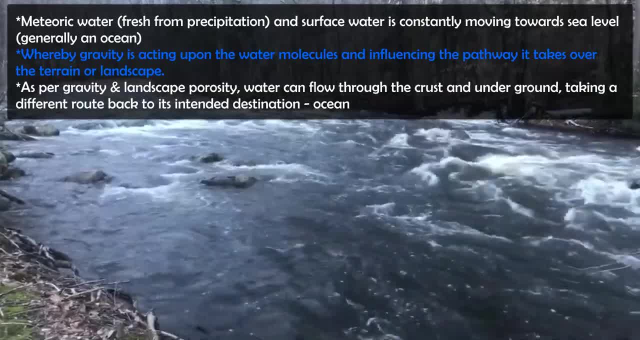 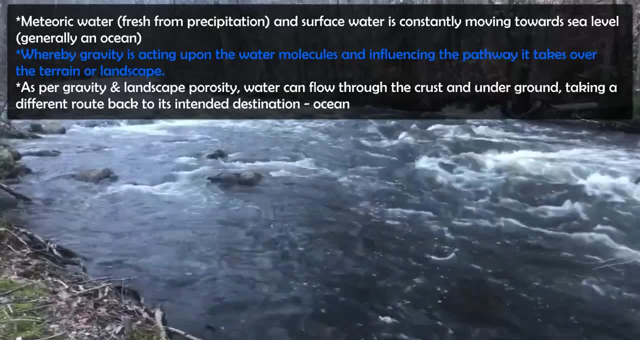 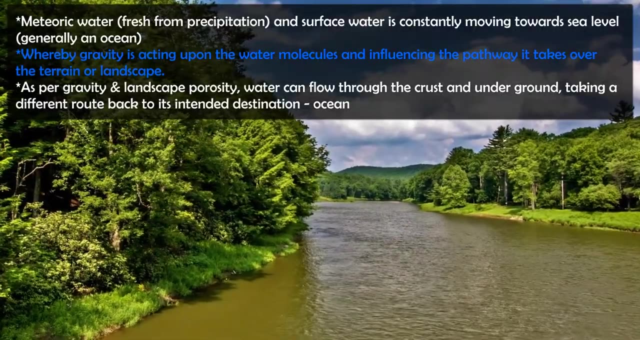 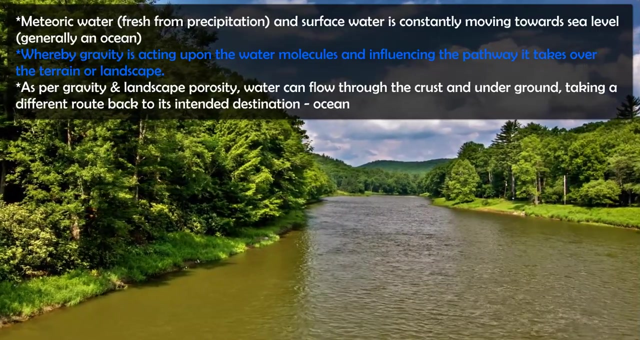 And, of course, you get the more calmer rivers that are based on certain stages of the river profile, which is more based on gradient, And they've lost The velocity of water and also on the the gravity that's pushing the water down. and you can get these meandering rivers going through low land or coastal areas on their way back to the ocean, which causes things like deltas to be produced, where water is going to combine and enter the oceans. 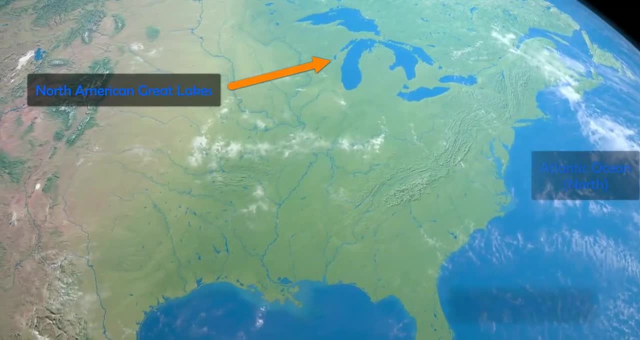 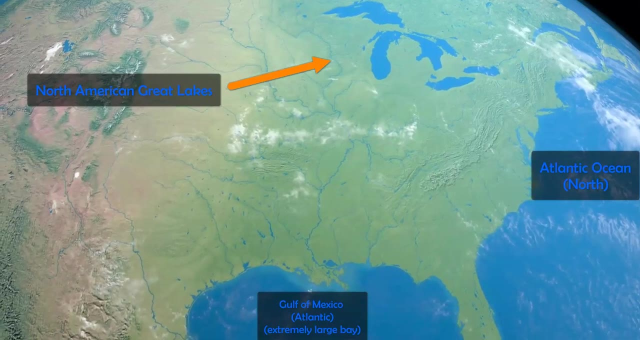 So from this aerial view, looking down on the lower 48 states of America, you see beautiful Mississippi River and the tributaries, the Missouri, the Ohio, these massive rivers flowing in And accumulating down in Louisiana into the Gulf of Mexico with the Mississippi Delta. 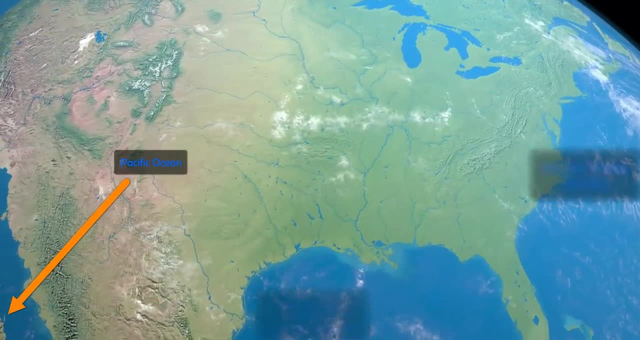 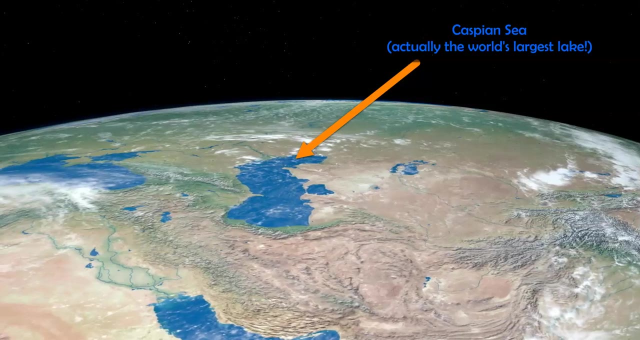 And you see how the carves are through from the high peaks of the Rockies to the left and the Appalachians to the right and how it comes in this massive drainage basin. Then we get the largest lake in the world, which is called the Caspian Sea in Asia. 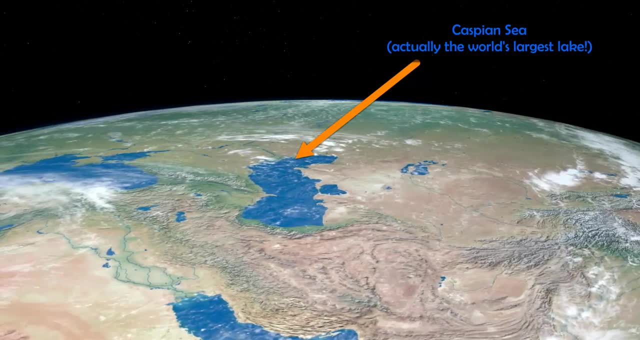 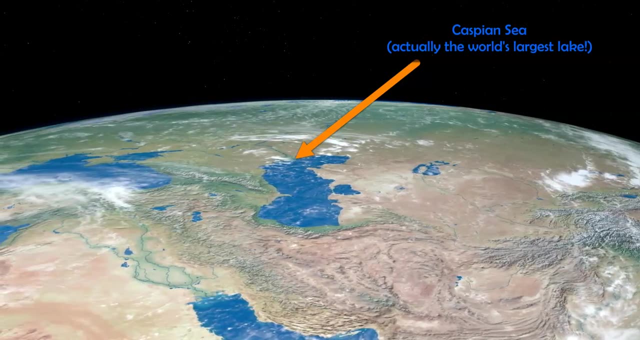 It's actually a lake because it is surrounded by land. there's no contact with the ocean. There are rivers that feed it in its lower depression, And the deepest lake is Lake Baikal, And the deepest lake is Lake Baikal. And the deepest lake is Lake Baikal. 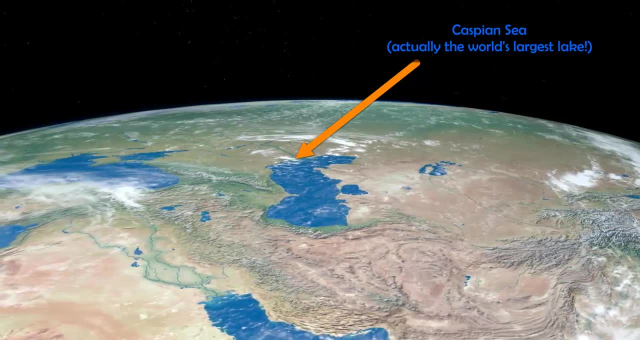 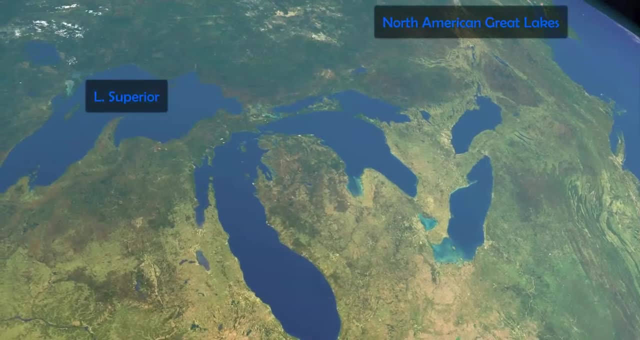 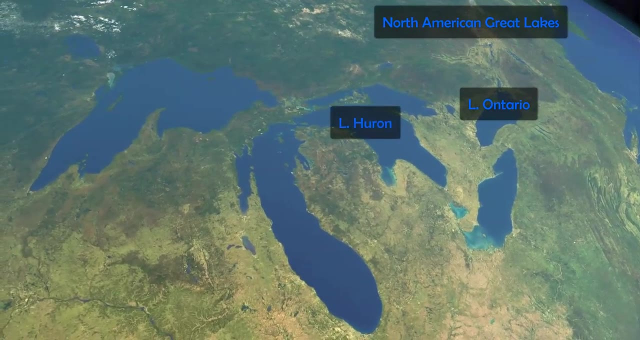 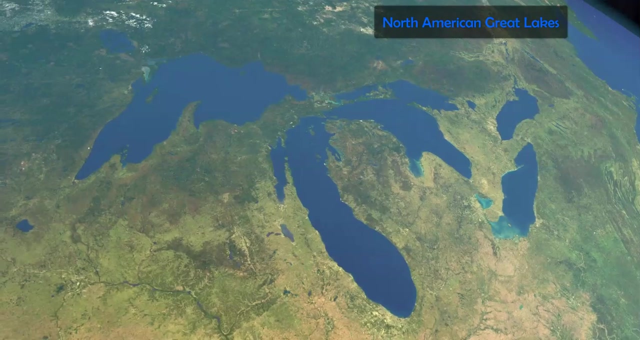